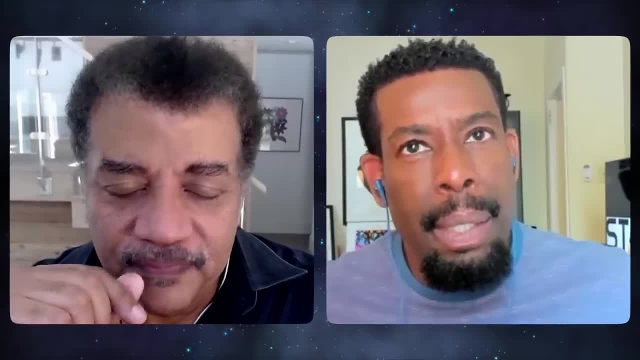 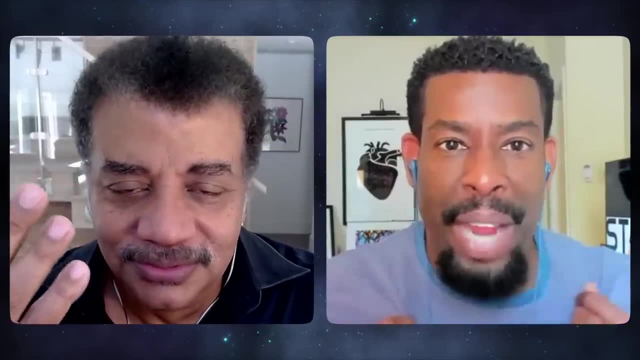 It can't warm. you Wait If you? Oh my God. Yes, You're right. Yes, But a sweater is not inherently warm. The sweater is just fabric. that's an insulator, really Correct. So if you are warmer than the outside and then you put on a sweater, it keeps your warmth. 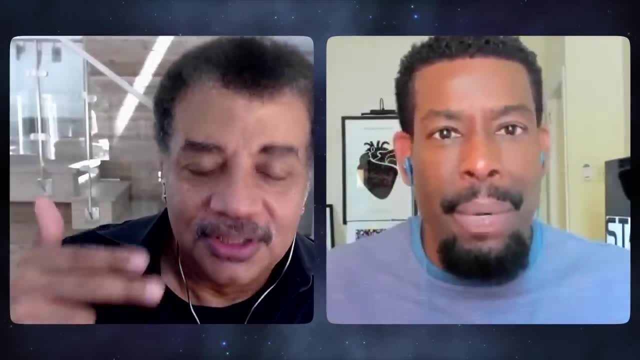 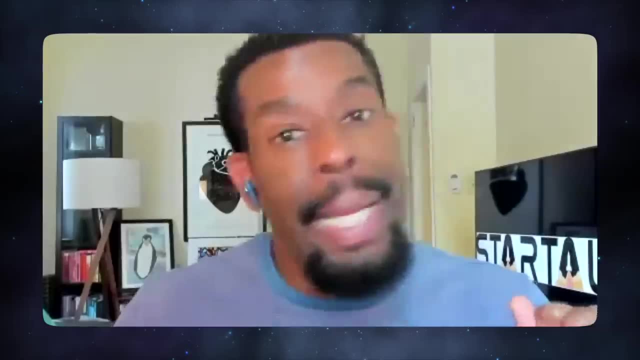 in you, Right, But if you are the same temperature as you all say, your clothing won't do anything. By the way, I do know- and I hate to say it and don't write- I know a couple of women who will put on a sweater when it's 98.6 degrees. 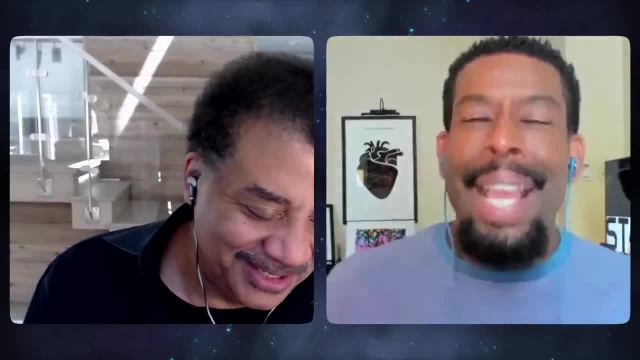 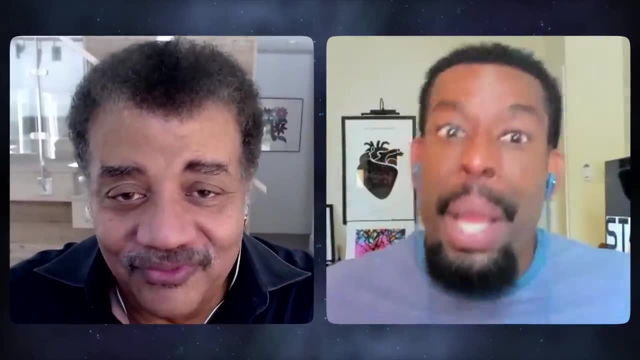 Really, Why is it so chilly in here? Don't stop. Oh my God, It's so cold. Okay, Yes, The thermodynamics of men and women have never been the same. Yes, You know, they did a study And they found that women are actually colder. 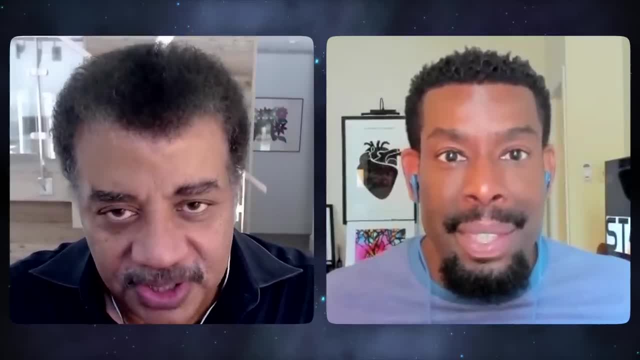 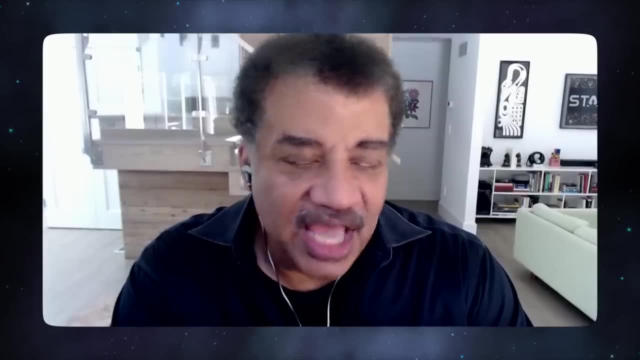 No, They did a study and found out that the temperatures in office buildings were specced for men because it was at a time when only men were occupying the office buildings, And so, yeah, the women end up colder. Had they specced it for women, men would be complaining how hot it was. 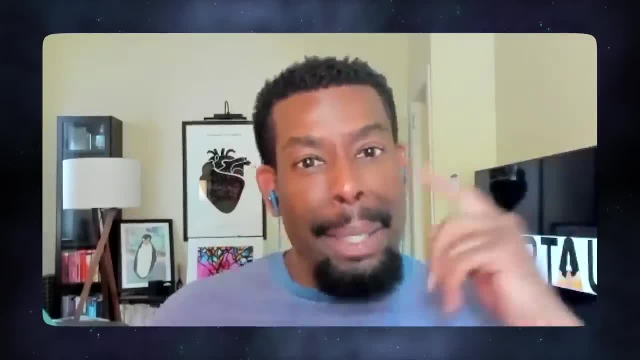 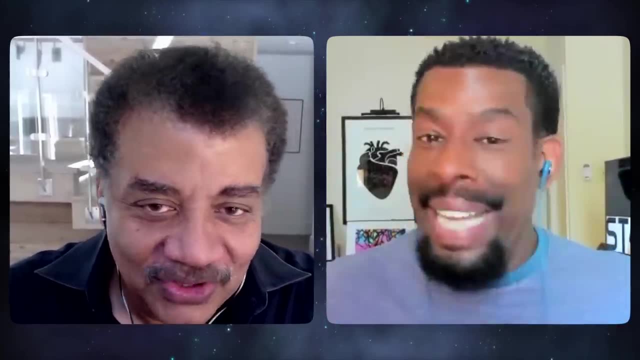 Okay, You're right, You know. That's why I'm glad I'm a man. No, I'm joking. Do not write. That is not. That's called a joke, That's it. Okay, Not right, Because I don't. 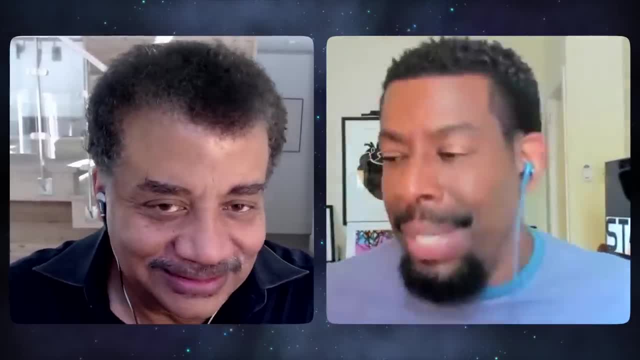 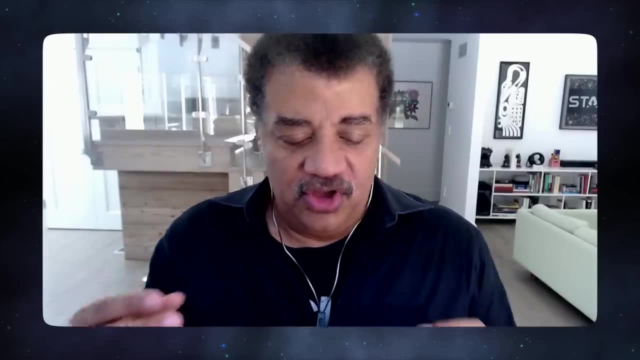 Okay, That would have rocked the house in 1987. It would have Right, You know, Let's get back. So these particles, you're lowering the temperature. Okay, So in quantum physics, every particle is also a wave. 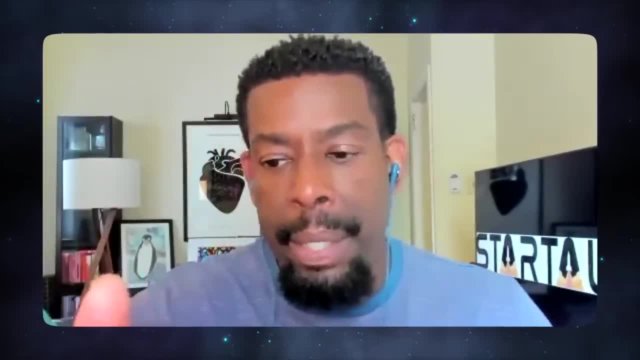 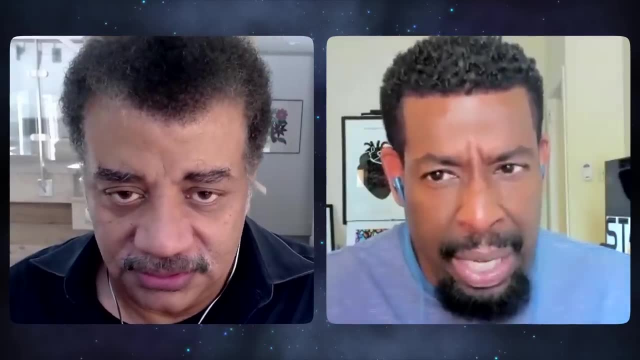 Okay, Holy Jesus, Give me a second man, Give me a second Quantum physics: every particle is also a wave. Now, is that because they're vibrating? It's? You want to ask rational questions. You want to ask rational questions. 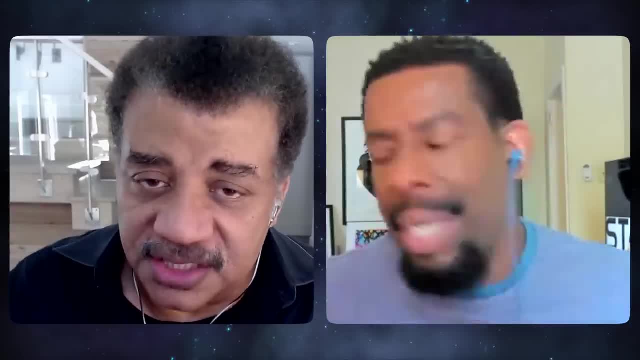 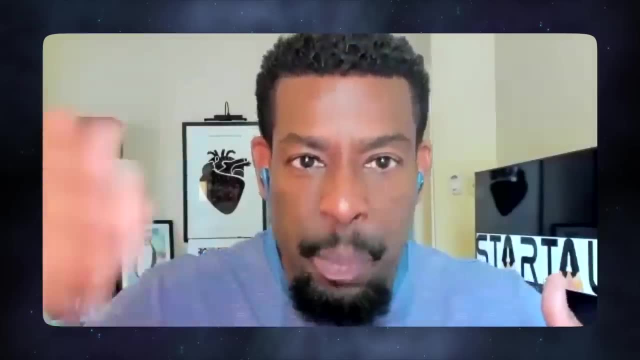 You want to ask rational questions about a reality that still transcends our common sense. Okay, Got you All right. So what you're saying here is like these are things you have to accept by suspending your natural understanding or your understanding of the world. 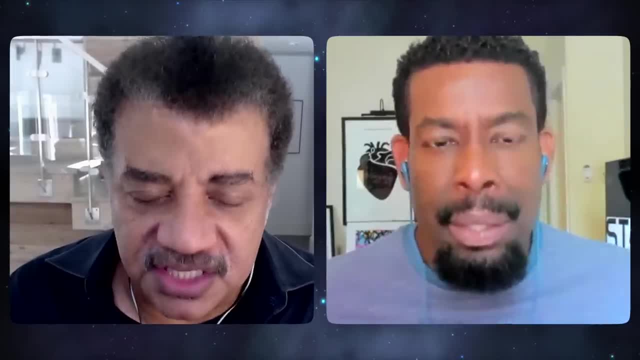 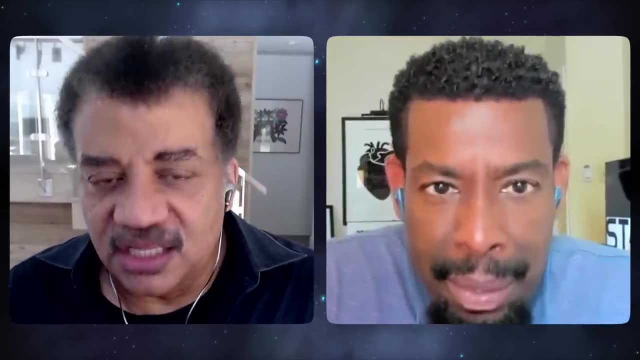 Your limited understanding, Your limited understanding Brought to you by your own five senses, Right Honed on the planes of the Serengeti to not be eaten by a lion, Right, All right. The universe is vastly more complex than that. 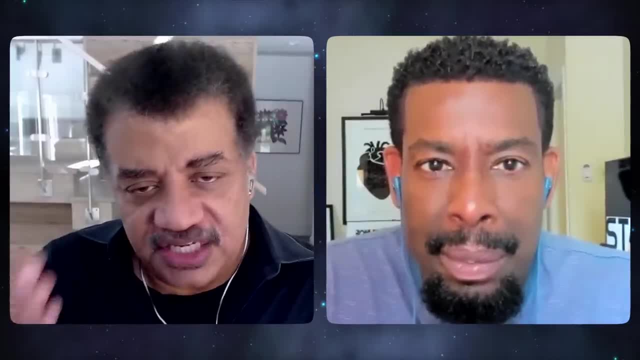 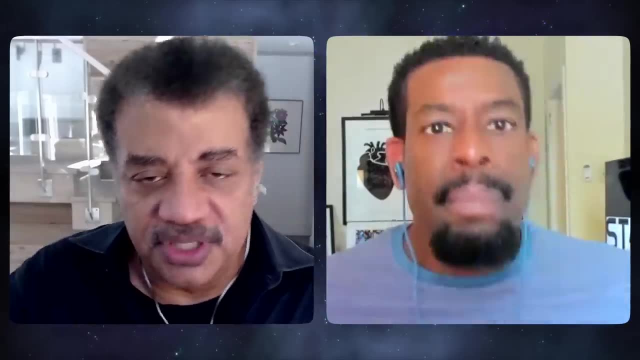 Gotcha And involves statements that, on the On the face of it, seem like they can't be true. Counterintuitive. That can't be true, But they are true Because your intuition is not quantum intuition, Right, It's classical intuition. 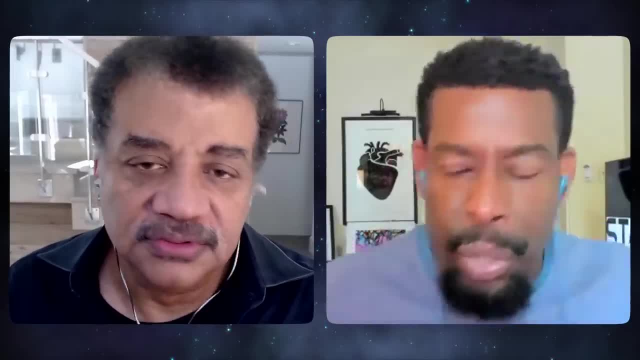 Right, Yeah, That's what I mean by your natural understanding. It's the world around you. Okay, Correct, All right. So now let's get back to this. Every particle is a wave on the quantum level. Okay, 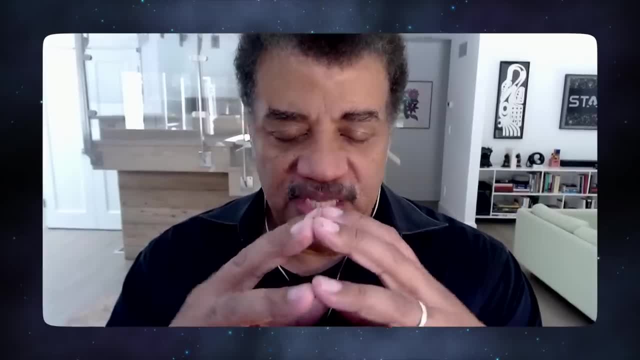 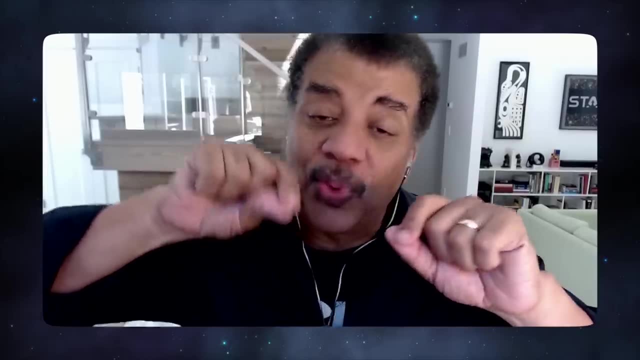 Correct, All right, And so on the quantum, it's also a wave, And so you have a jumble of particles and they're all doing their thing. You can look at what wave is associated with them, What wavelength, Length: 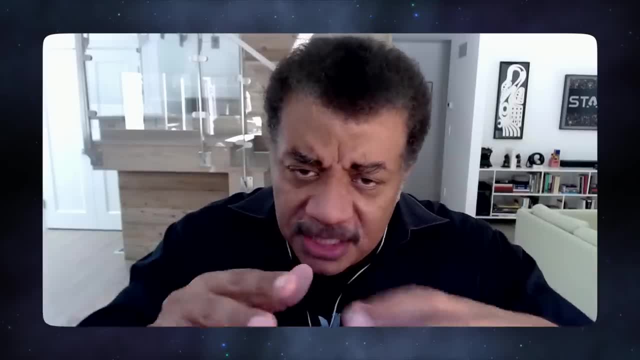 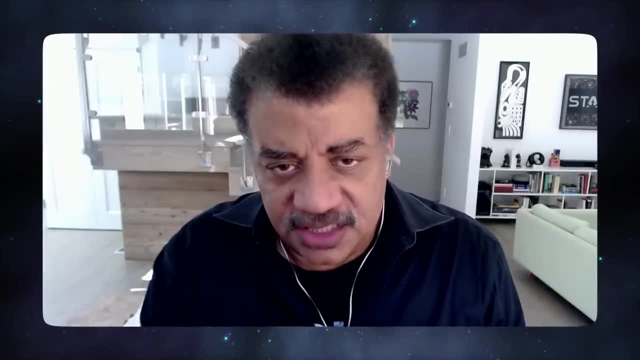 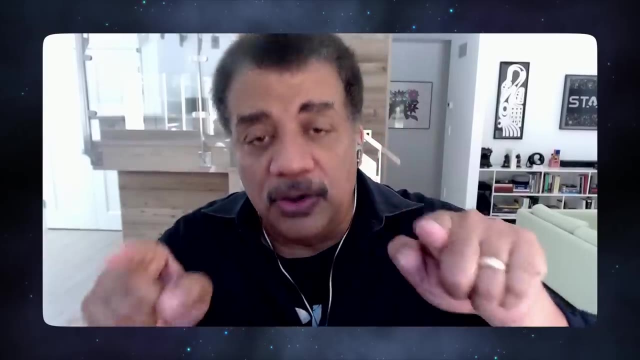 Okay, And they're each doing their thing. Mm-hmm. They're all independent particles, Okay, So let's cool them down, Mm-hmm. As they vibrate less, they have less energy associated with them and their wavelength grows. 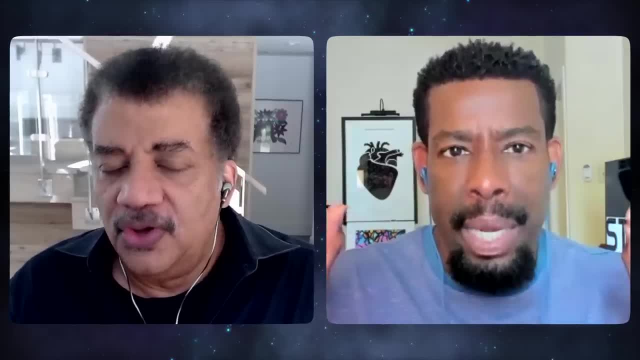 Aha, Okay, Okay, All right. So just hang with me. now I got you. I don't want to lose you. Okay, I'm with you right now. Right now I got you. Okay, Okay, Okay. 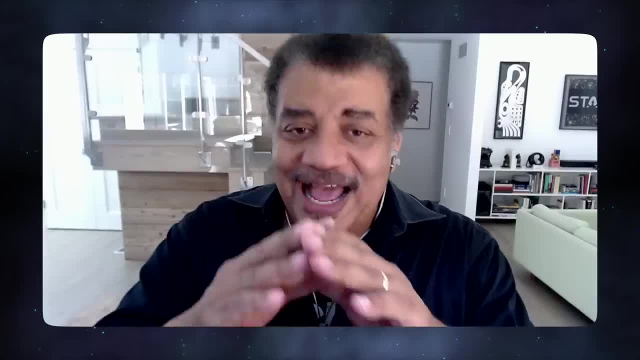 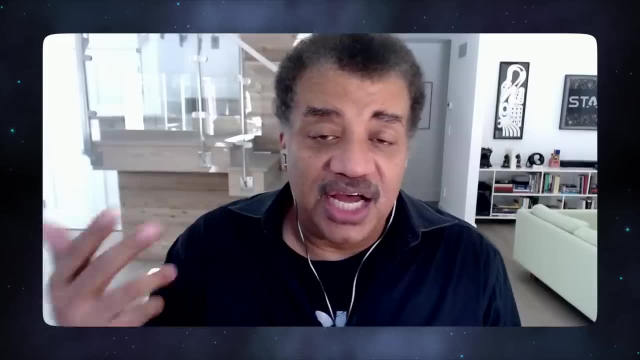 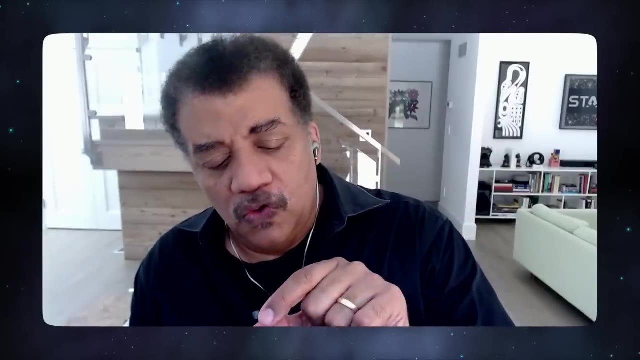 Okay, Okay, Okay. So the characteristic wave of the particle, as it slows down, begins to grow. Right, Okay, Now there's what's called the Heisenberg Uncertainty Principle. Oh, Okay, All right, Which is: the more you know about a particle's position in space, the less you know about. 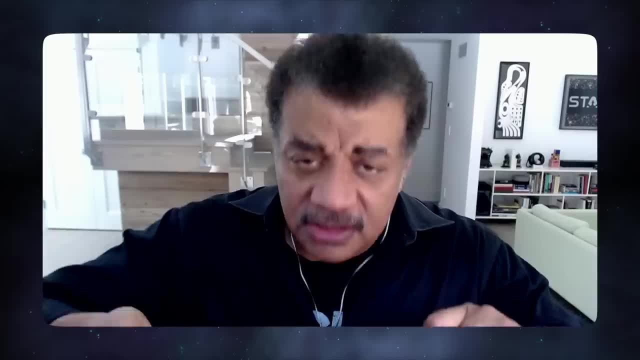 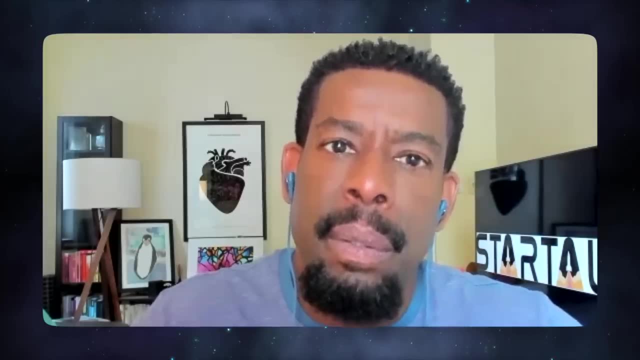 its energy, And the more you know about its energy, the less you know about its position in space. Okay, Okay, Okay. Now there's a geeky way to get out of a speeding ticket, where the cop stops you and it says: 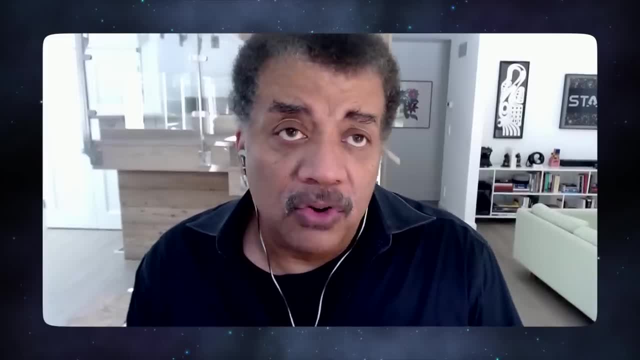 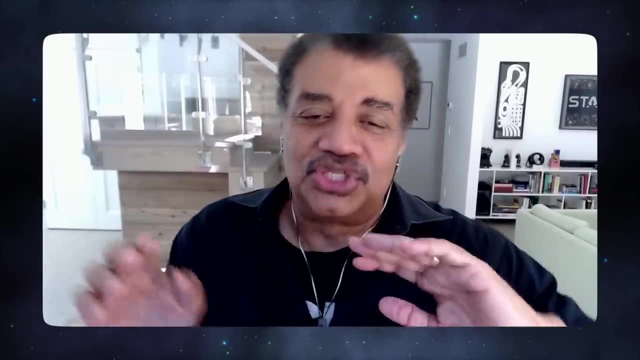 do you know how fast you were going? And you just say, no, that means I'm everywhere or something. There's some stupid quantum. okay, that's surely to get the black man shot. and then There you go. That's how that works. 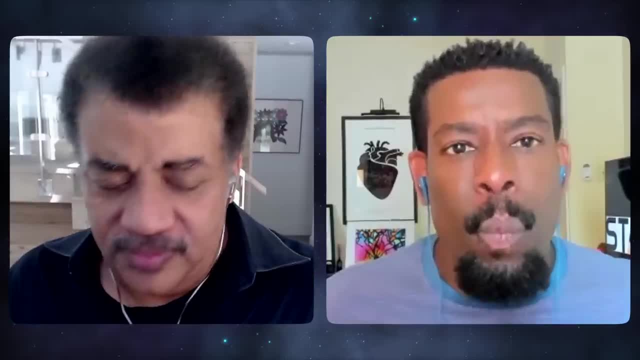 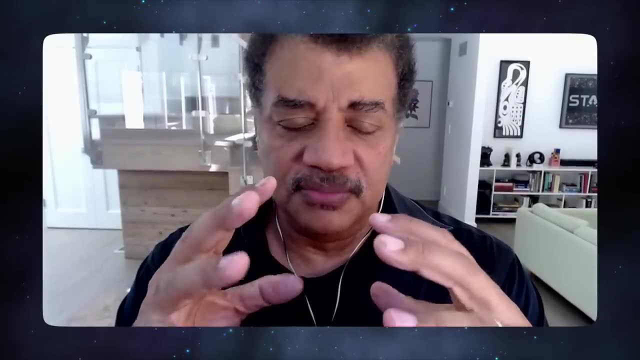 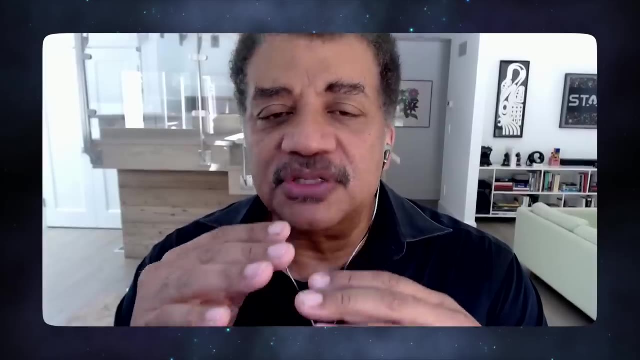 That's how that works, All right, So, anyhow, Okay. So you have these particles And as you cool this material. when I say cold, I don't mean put it down in the freezer. I'm talking on a Kelvin absolute temperature scale, where zero is the coldest. 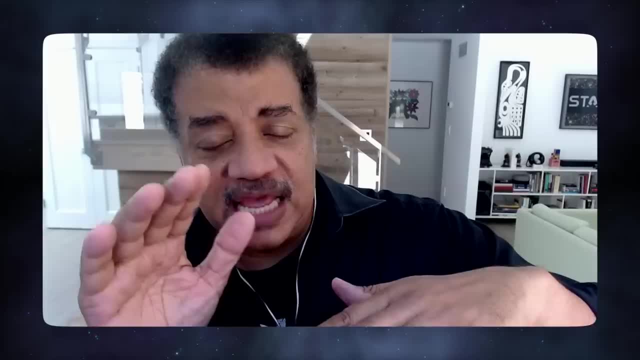 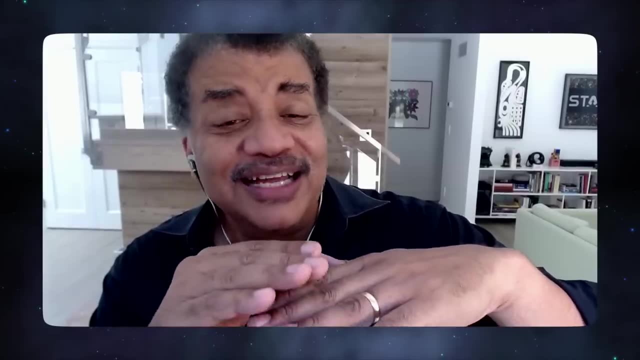 We have a whole explainer on that one. Yes, we do, I remember. Yes, You can get down to 10 degrees and nine, eight, seven, six, five, four, three, two, one, a half a degree, a tenth of a degree, a thousandth of a degree. 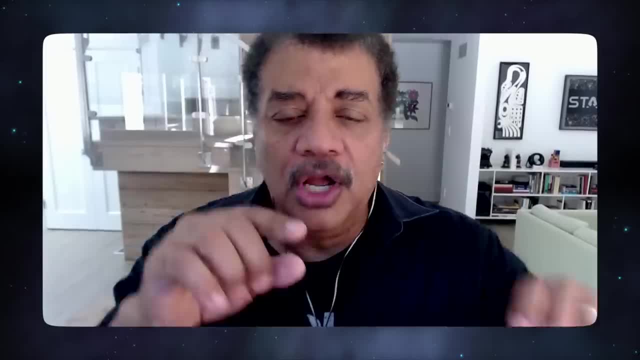 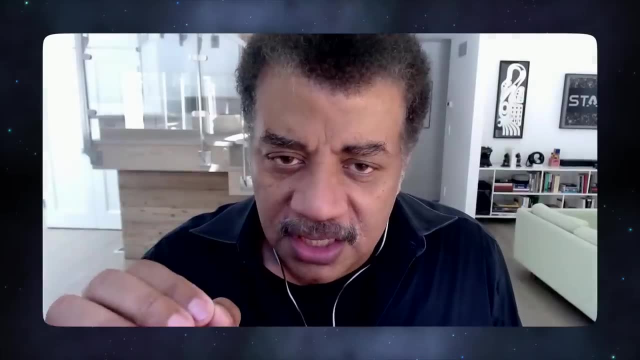 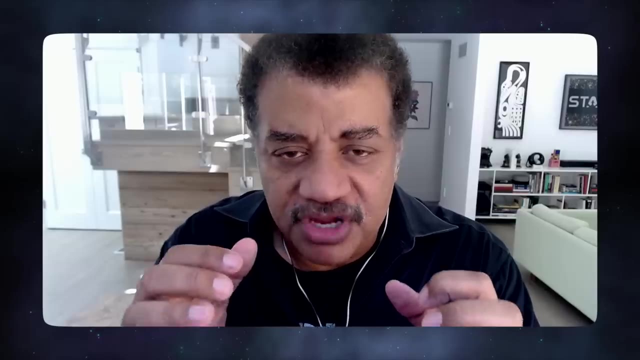 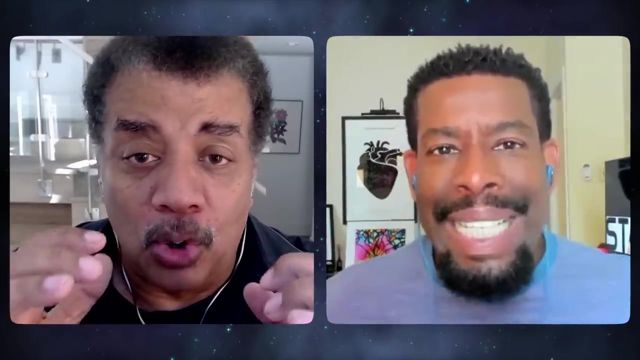 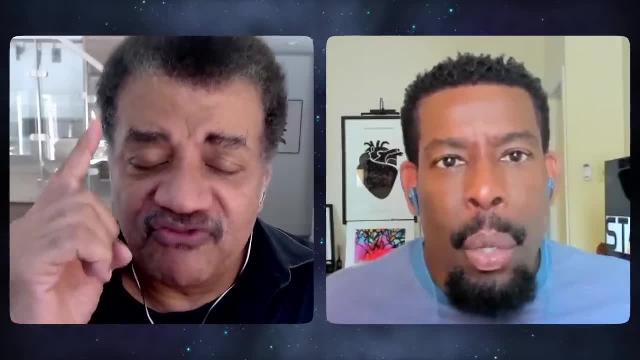 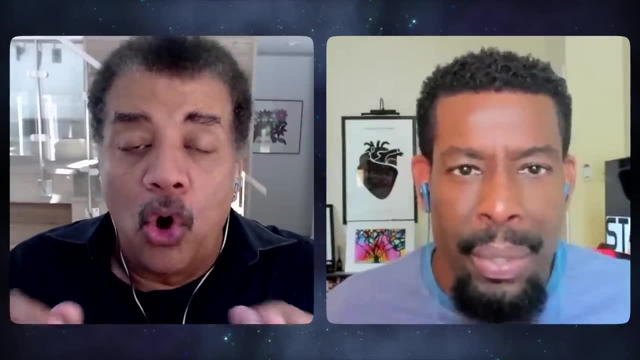 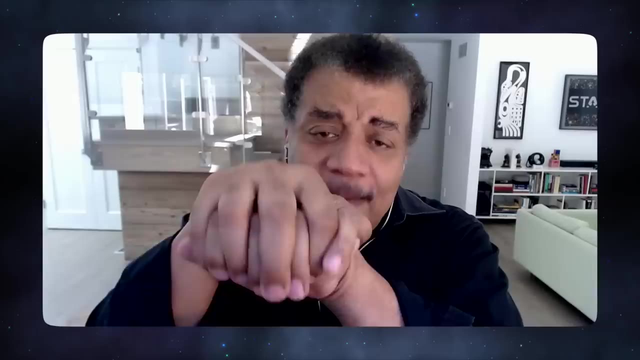 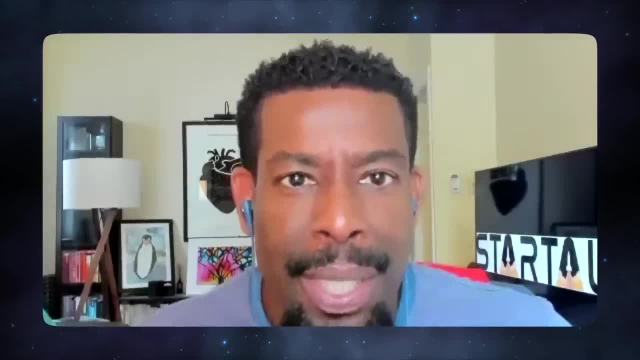 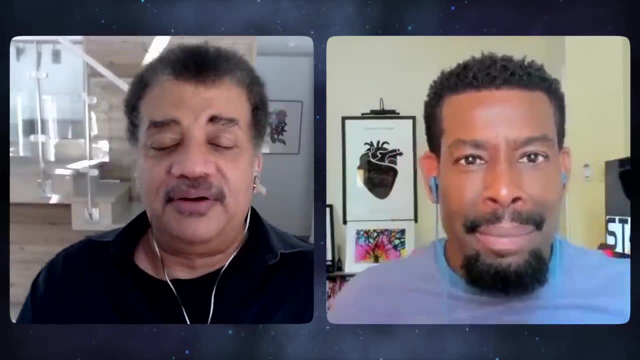 with each other. They're the Voltron of particles. Okay, I forgot who Voltron is. Who's that? That's the one where all the little robots come together to make one big giant robot. Yes, There it is. There it is. 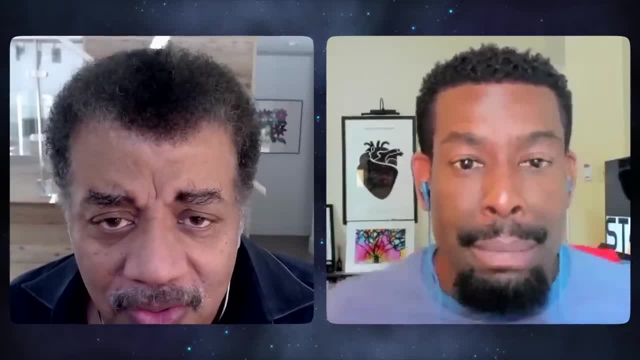 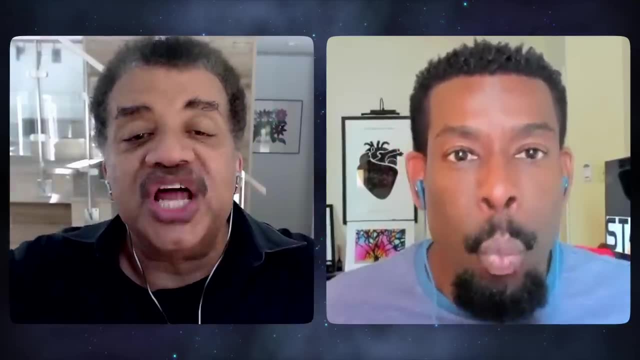 What movie was that? What comic book was that? Voltron- Oh, Voltron is the story. Yeah, That's the story. Okay, That is it. Yeah, So all the particles come together and they become one metaparticle. 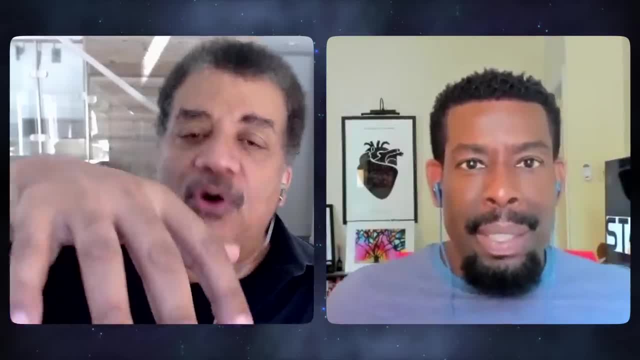 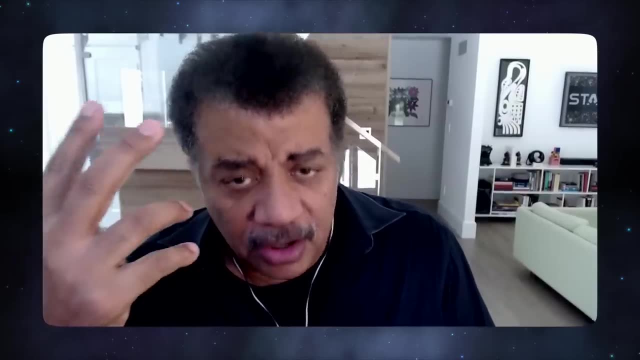 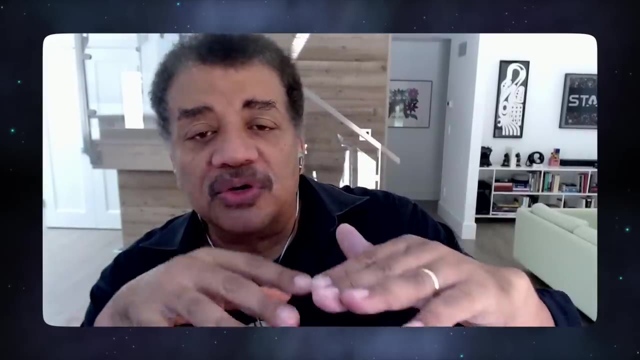 One, A functioning metaparticle. Correct, Because they all resonate together at the same time. Sweet, And this is why you can't think of matter as only particles or waves, All right, Because, depending on the situation, they will function as one or the other. 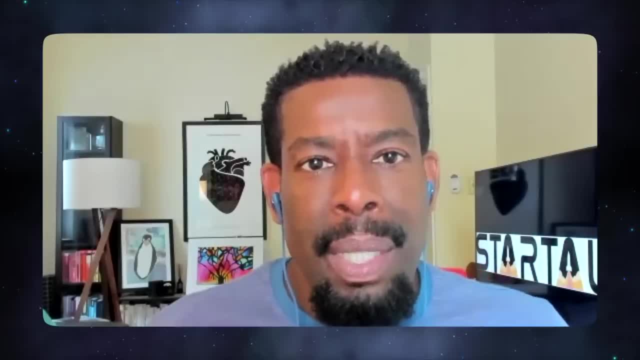 And in some cases both Wow And so oh yeah. And, by the way, there's a lot of phenomena, So that's a Bose-Einstein condensate. It happens like quick. As you drop the temperature it transitions. 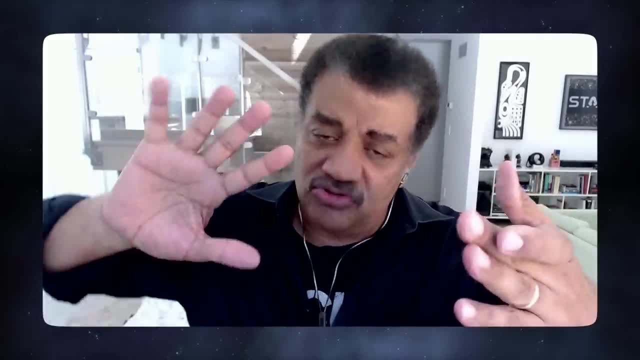 Boom. It's basically a phase change in what it is. It's weird for us to think that, But is it really any weirder than having a transparent liquid all of a sudden become solid? Right, Not really. Think about it. If you've never had a transparent liquid, it's not going to be solid. 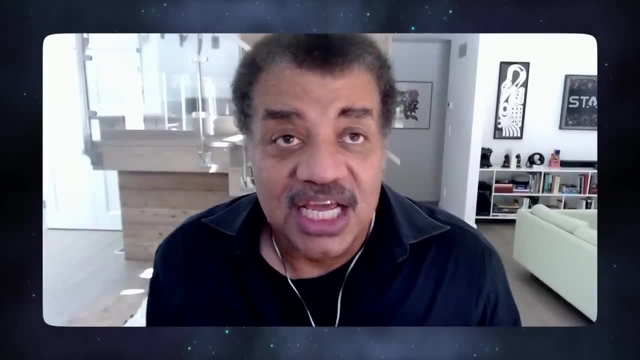 Right, Not really. Think about it. If you've never had a transparent liquid, it's not going to be solid Right, Think about it. If you've never had a transparent liquid, it's not going to be solid Right. 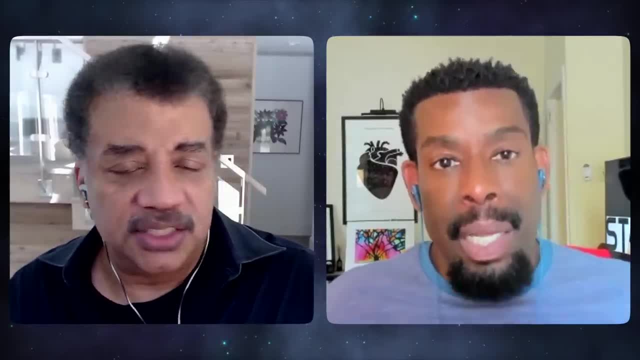 If you've never been in a freezing temperature and someone has a- A cube of ice, A cube of ice, And you say what's that? It's water. And you say, no, it's not, because I can't drink it. 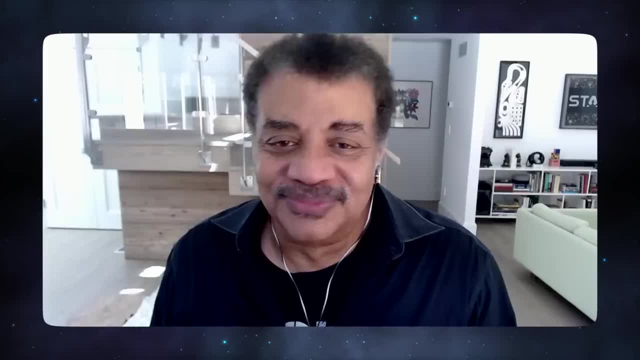 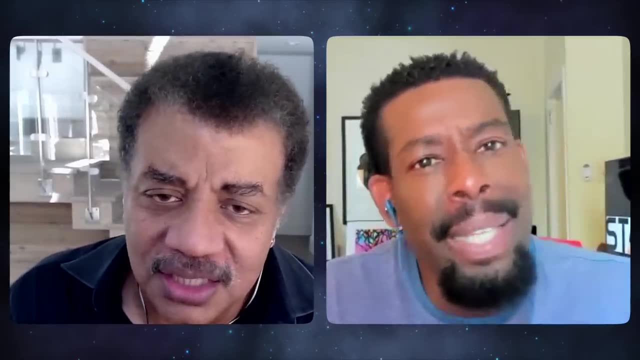 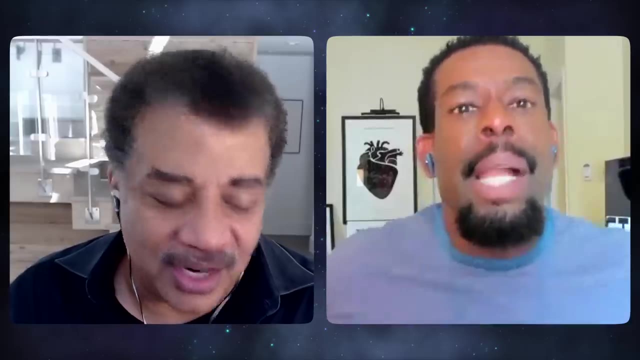 And it's not a liquid, And it's not- Witch, Witch. Now why do they only burn the witches and not the warlocks? You know, why did they never find the warlock, is the question. So the men had all the power, I guess. 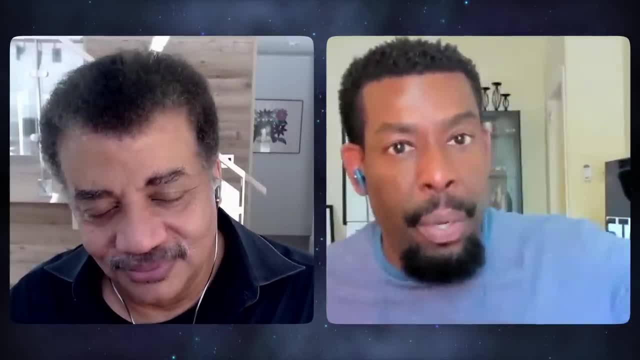 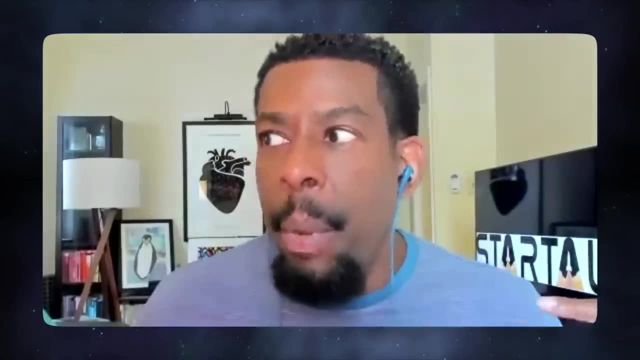 Which I don't understand, why every woman, the person who, ever- because it's always- It's always a guy, right, You know, Witch? And immediately, if I was a woman, I'd have been like: yes, I'm a witch. 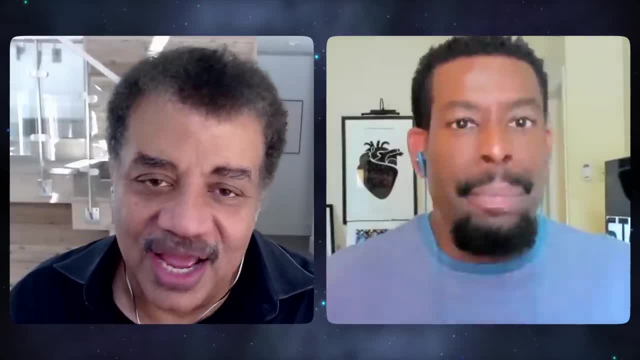 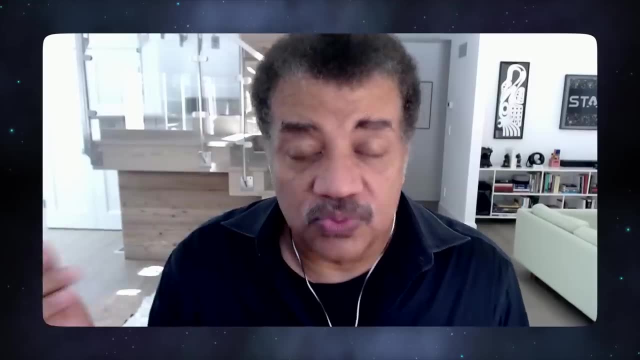 He's my warlock. Oh yeah, Yeah, Yeah, Totally, take that one out. Yeah, We're going down together, baby, Fight the fire with fire. Fight fire with fire, Yeah, Yeah. So other phenomena like this. one of them is called super fluidity. 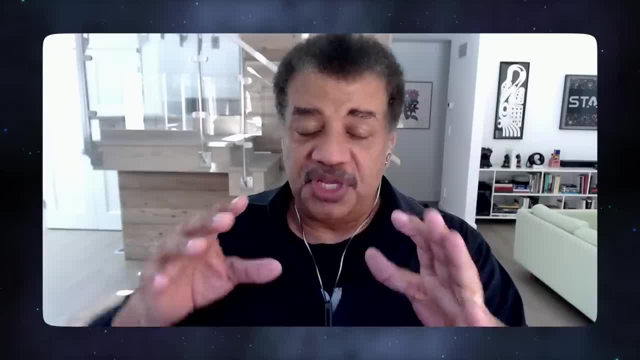 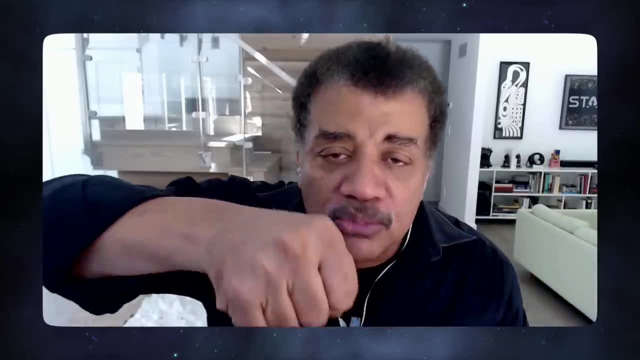 You know what that is. The fluid becomes a super fluid, which means if you pass something through it like your fist- Right, There is no resistance to your hand moving through it. Through that volume, It just envelops your hand as though nothing is there. 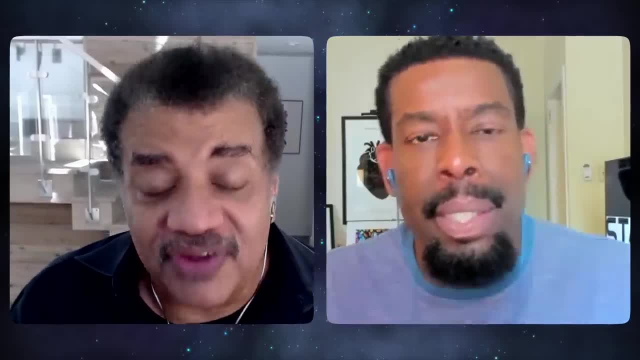 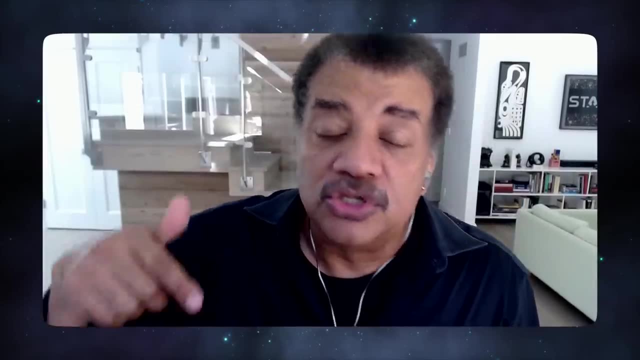 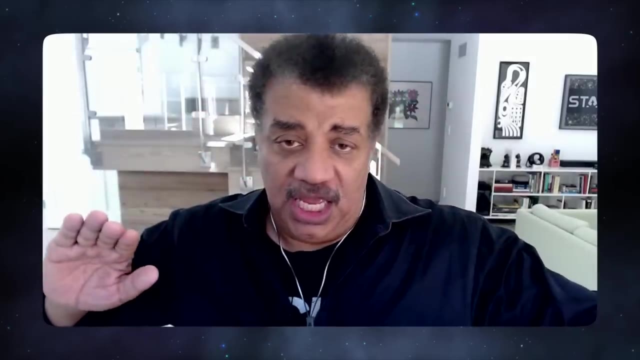 It's super fluidity, That's a- Then you can have super conductivity, where the material offers no resistance to the movement of electricity, So you don't lose any electric power to heat, okay, And you have perfect transmission of electricity, And so you can have super conductivity and from that you can get super conducting magnets. 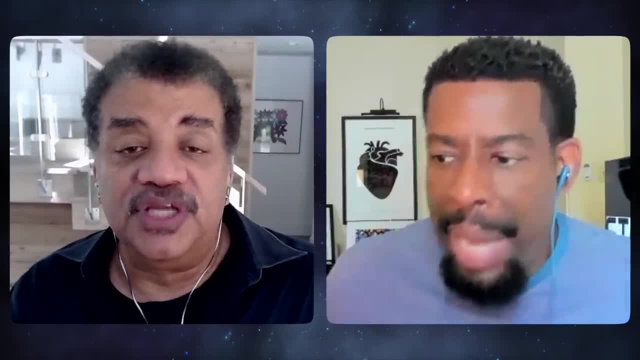 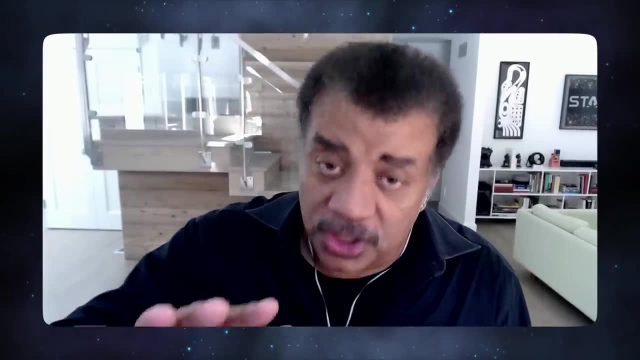 which are extremely powerful. That's the levitating magnets. Yeah, Yeah, You get some of that. You get some of that. Okay, Well, you get a maglev train that would help out. It could be totally happening if you can get super conducting magnets to do that. 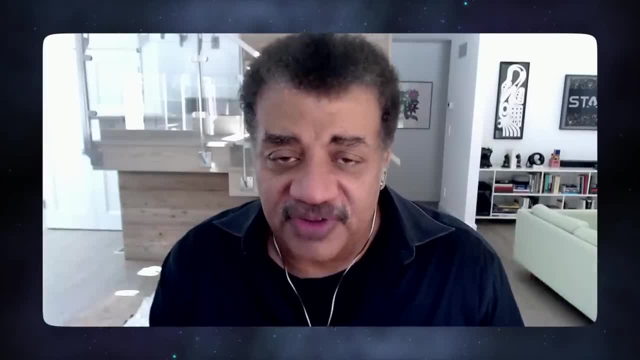 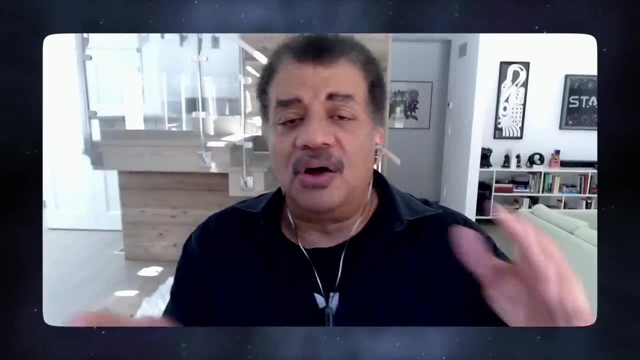 The problem is you can't cool everything to fractions of degrees above Kelvin. You need sort of high temperature, super conductors, high temperature which would still be very cold, And so it's a whole thing. It's a whole frontier in material science and in physics. 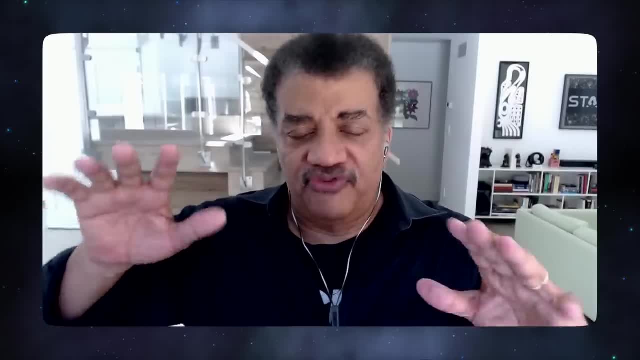 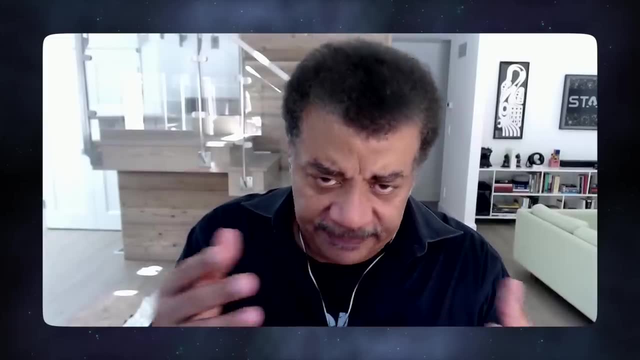 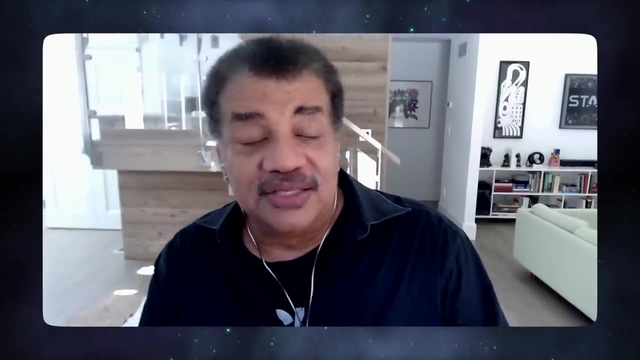 Wow. So the point is, none of these phenomena make any sense in a classical world, Right, But when you bring in quantum forces and put it under those conditions, you need quantum physics to understand it, And so I just think it's cool that all these particles can condense and act as one meta. 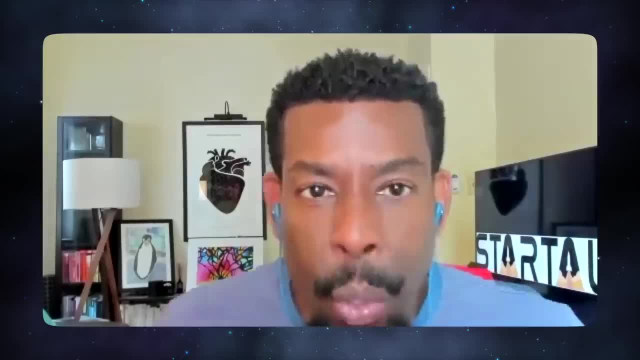 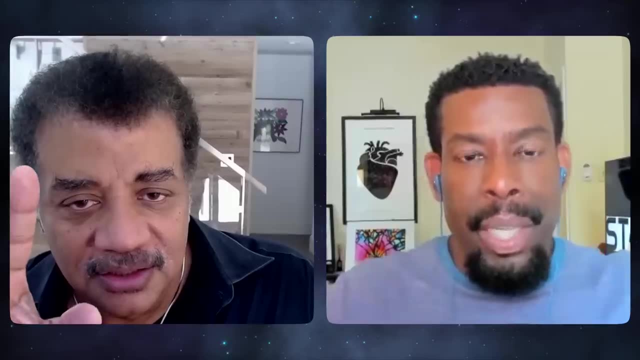 system And you said: it's not Ultron. Who was it, Did you say- Voltron. Voltron, It's the sum of smaller robots that's acting as a single robot, As a single robot. Yeah, Voltron is a Bose-Einstein condensate. 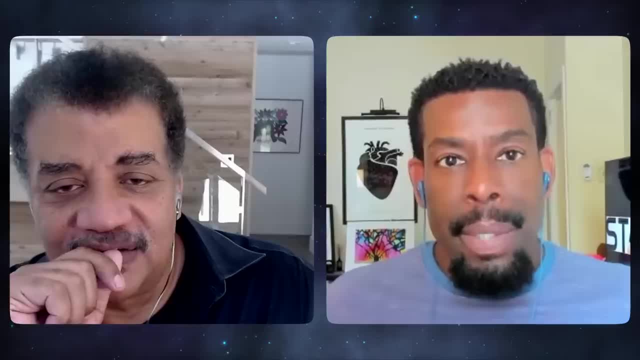 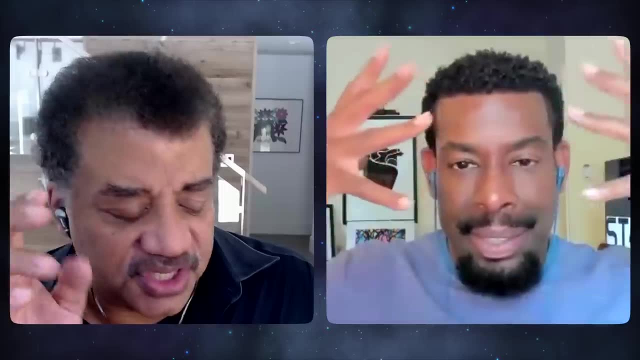 Look at that, That's pretty awesome. Yeah, That's right. So there it is. That was quick. No, it was great. Yeah, I did not-. We need a healthy respect for quantum physics as we enter the realm of quantum. 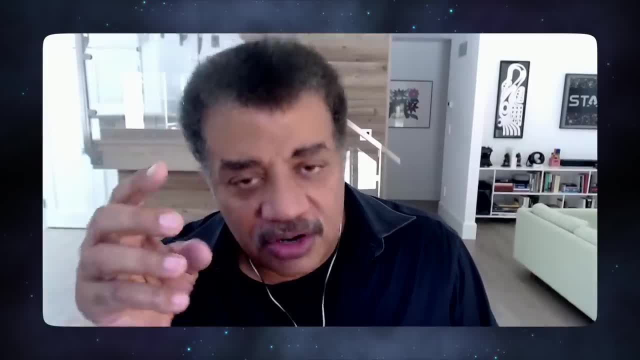 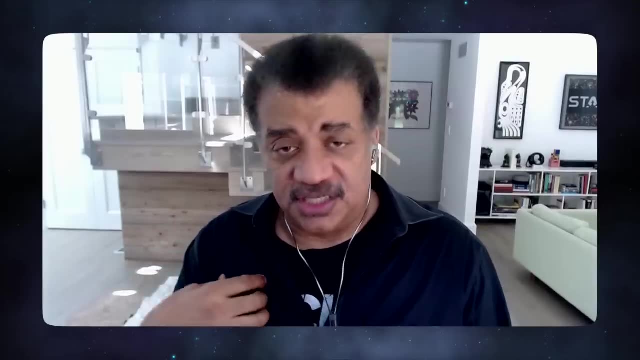 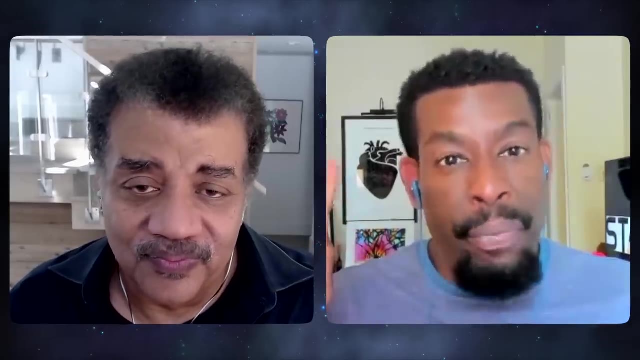 computing, where once again, we exploit the weird wacky stuff that is normal in quantum physics and is out of our life experience, from our senses. And so there it is, Chuck. Okay, That is super duper fly. No, it's super duper conducting. 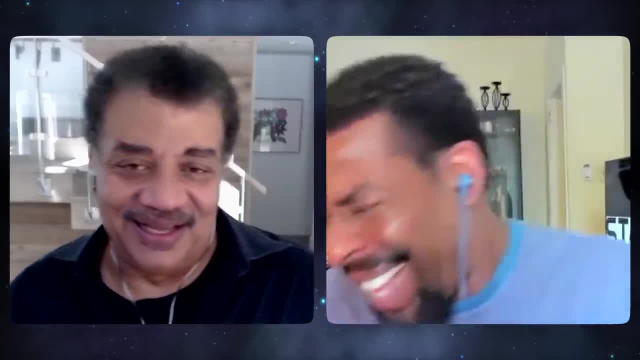 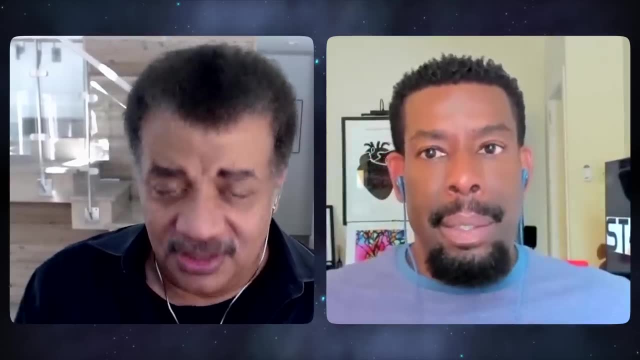 Oh, by the way, speaking of super duper- Yeah, We're going to build the world's largest particle accelerator, And you know how you accelerate particles? Okay, You get a particle with a charge in it and then you shoot it into a magnetic field. 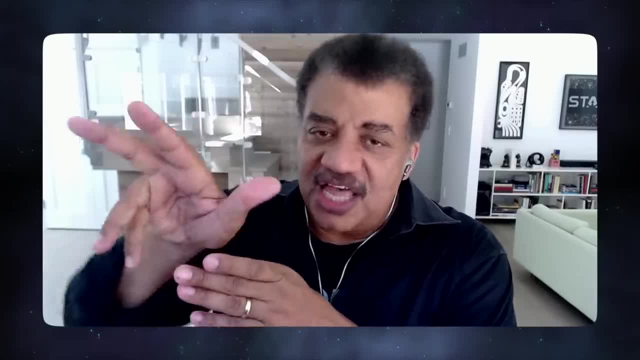 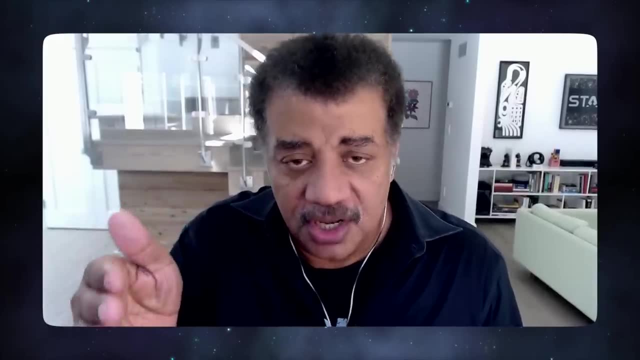 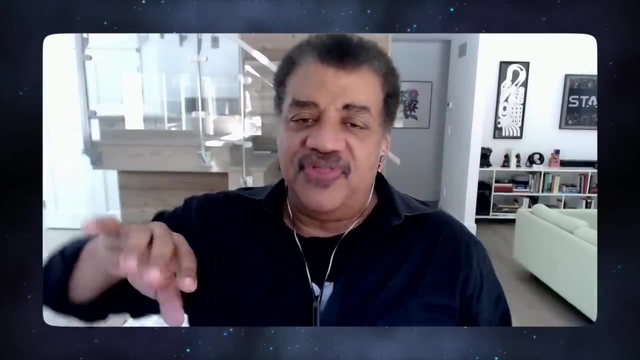 Okay, And if you vary that magnetic field you can accelerate the particle. But the particle wants to have its direction of motion changed. It starts arcing, So you know exactly how much it's going to arc. You make a tube that's round and then you alter the magnetic field in that tube to accelerate. 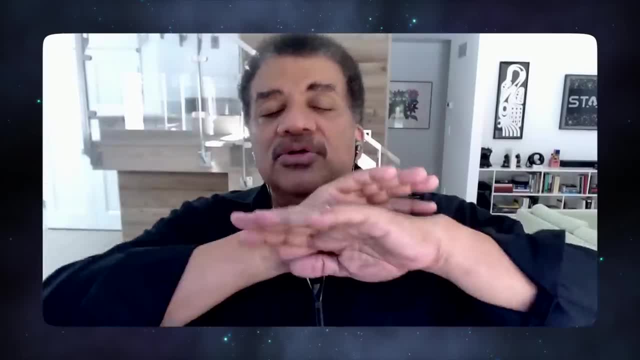 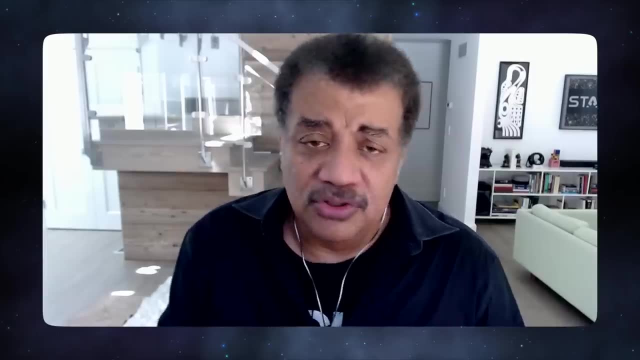 the particle. This is how every single circular particle accelerator works. Okay, And you can only accelerate particles that have charges. You can't accelerate neutrons. You can't accelerate neutrons because they don't have charge. Okay, That's that joke in the bar. 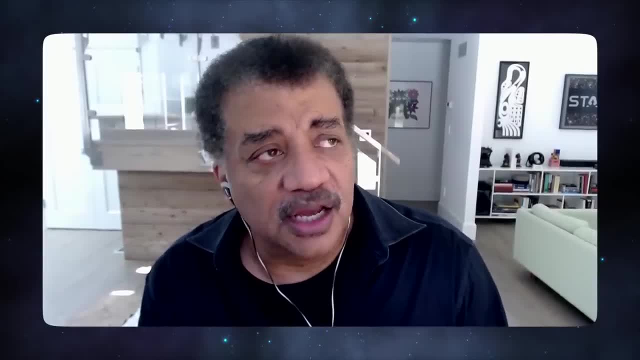 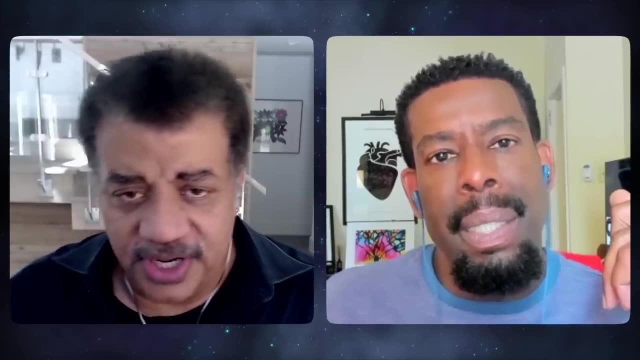 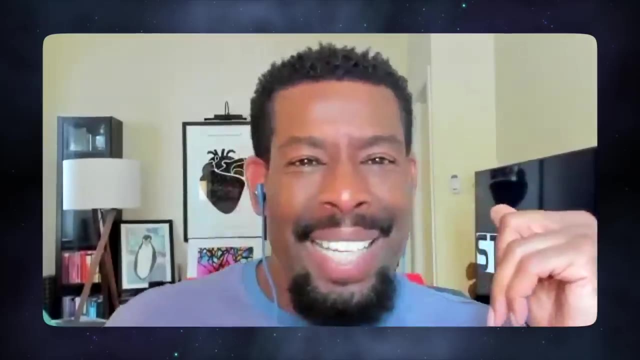 Neutron walks into a bar and says I'd like a beer. So here it is, And the neutron says how much? And the bartender says: for you, no charge. That's stupid, Stupid. So, just as we go forward, just embrace all that quantum physics brings you and don't.